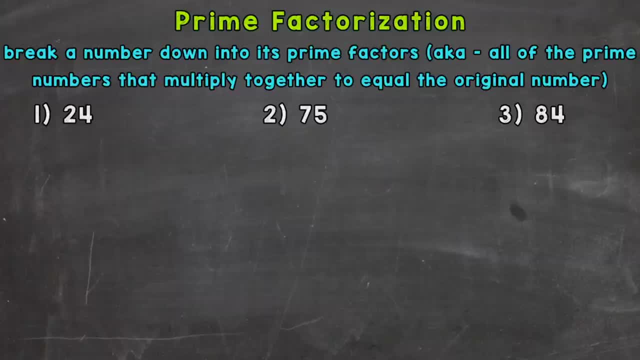 one and the number itself. Now, the opposite of prime is composite, so numbers that have more than two factors more than just one and the number itself as factors. If you need a little review on prime and composite numbers, I have a video that goes over those two things down in. 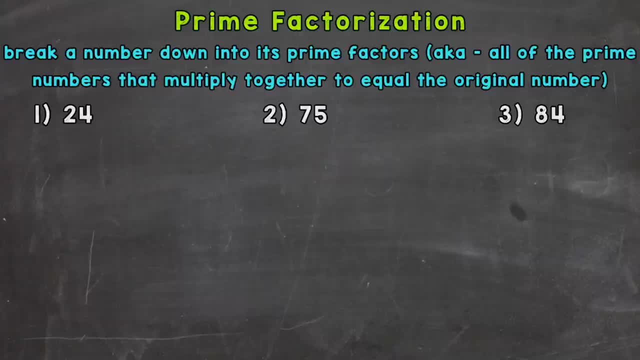 the description. So let's jump into number one, where we have 24.. And we need to start by breaking this down into any factors of 24 that we can think of. So let's think of two factors of 24.. For example, 2 and 12 are factors of 24.. 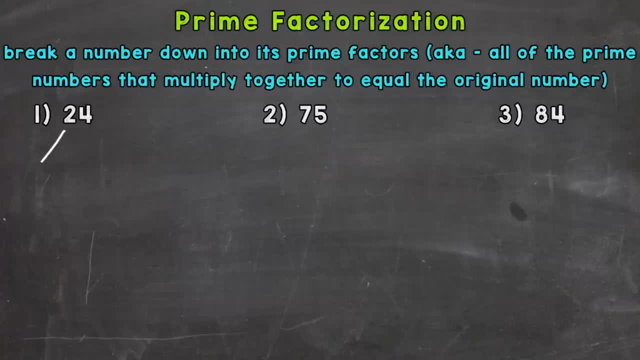 So let's break it down: 2 and 12.. Now 2 is a prime number, so our path ends there as far as that side, 12 is composite. so we can keep breaking 12 down until we get all prime numbers. So let's. 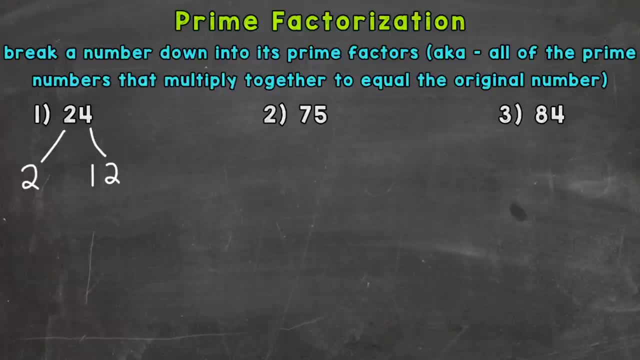 think of some different factors of 12 in order to continue breaking it down. So we know: 6 times 2 equals 12.. 6 and 2 are factors of 12.. Now 2, right here, this 2 is prime, so that path ends there, But 6 is composite. We can continue. 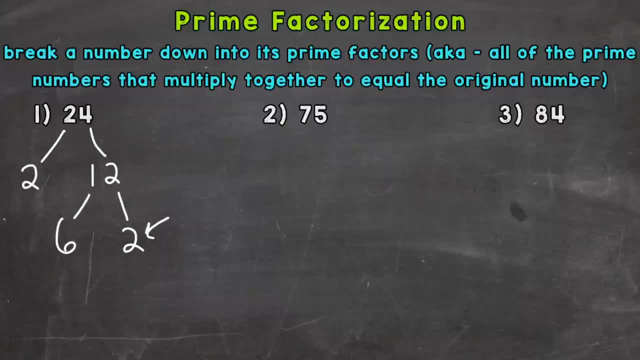 on until again, all prime numbers. Well, we know, 3 and 2 are factors of 6.. So 3 times 2 equals 6.. And there we go: 3 is prime and 2 is prime. So we have all prime numbers here: 2,, 3,, 2, and 2.. 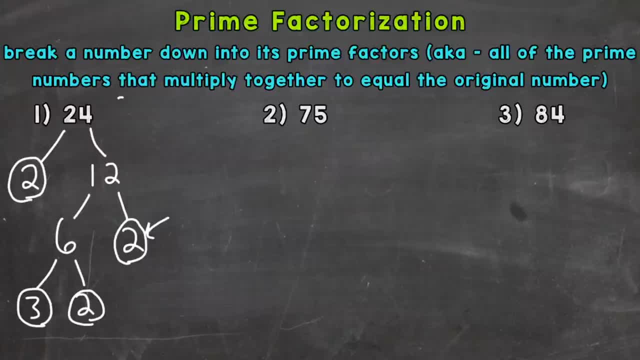 If we have it correct, those will all multiply to equal our original number of 24.. So we get the answer of 2 times 3 times 2 times 2.. So 2 times 3 is 6.. Times 2 is 12.. Times 2 is 24.. So that's. 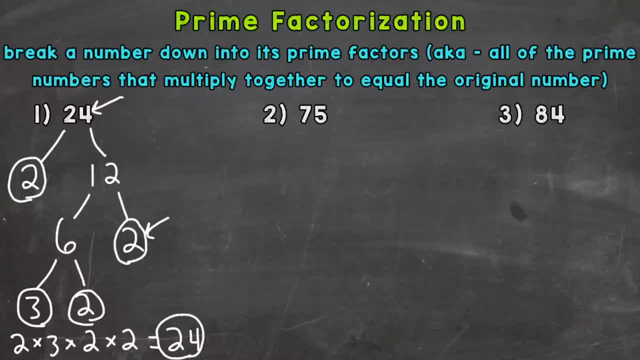 the prime factorization of 24.. Now I do want to show you that there are multiple paths, So let's zoom in real quick and see if we get the same answer. So I'll try to squeeze it in here: 24,. well, I know 6 and 4 are factors of 24, but both of those are composite, So we can continue on. 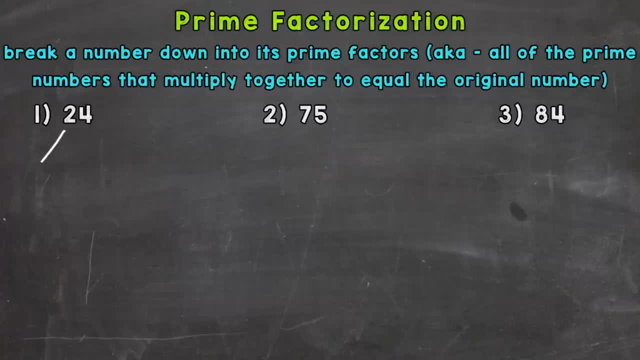 So let's break it down: 2 and 12.. Now 2 is a prime number, so our path ends there as far as that side, 12 is composite. so we can keep breaking 12 down until we get all prime numbers. So let's. 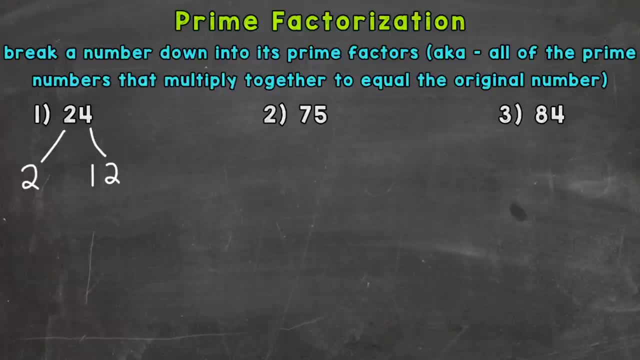 think of some different factors of 12 in order to continue breaking it down. So we know: 6 times 2 equals 12.. 6 and 2 are factors of 12.. Now 2, right here, this 2 is prime, so that path ends there, But 6 is composite. We can continue. 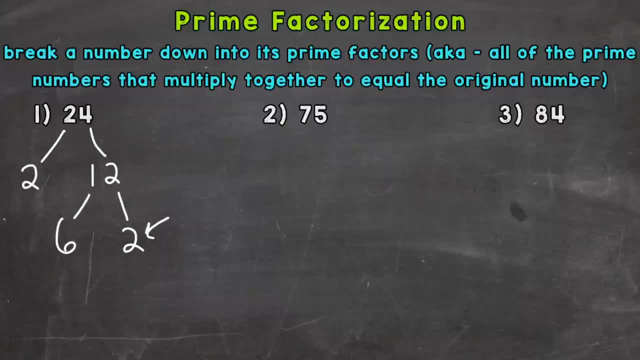 on until again, all prime numbers. Well, we know, 3 and 2 are factors of 6.. So 3 times 2 equals 6.. And there we go: 3 is prime and 2 is prime. So we have all prime numbers here: 2,, 3,, 2, and 2.. 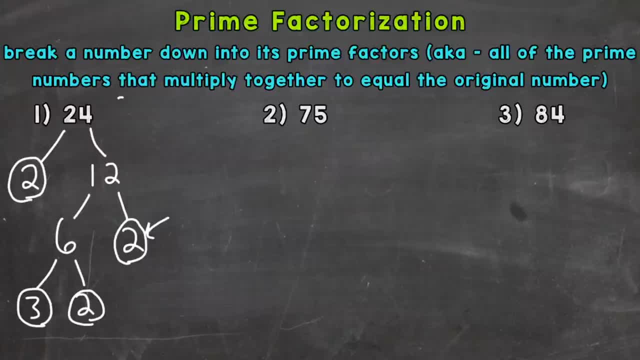 If we have it correct, those will all multiply to equal our original number of 24.. So we get the answer of 2 times 3 times 2 times 2.. So 2 times 3 is 6.. Times 2 is 12.. Times 2 is 24.. So that's. 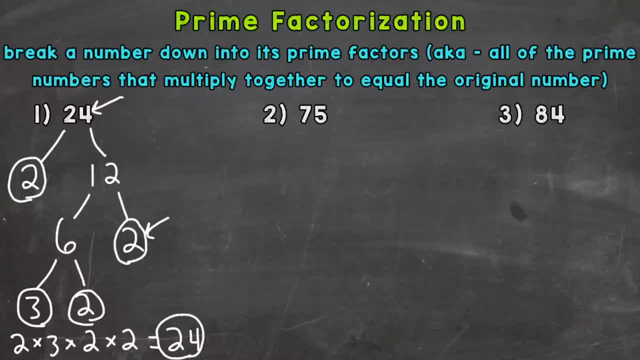 the prime factorization of 24.. Now I do want to show you that there are multiple paths, So let's zoom in real quick and see if we get the same answer. So I'll try to squeeze it in here: 24,. well, I know 6 and 4 are factors of 24, but both of those are composite, So we can continue on. 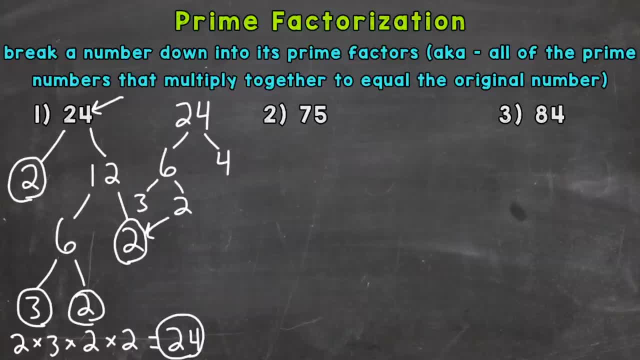 Well, 3 and 2 here for 6, factors of 6.. And then 4 would be 2 and 2.. So we get 3,, 2,, 2, and 2.. So the same exact answer, but a different path. 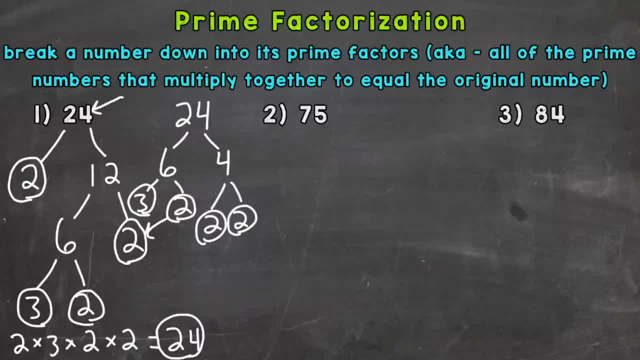 And in number 2, where we have 75. So we need to think of a couple of factors here to begin breaking this down to its prime factorization. Well, we know, 3 times 25 equals 75. So 3 and 25. 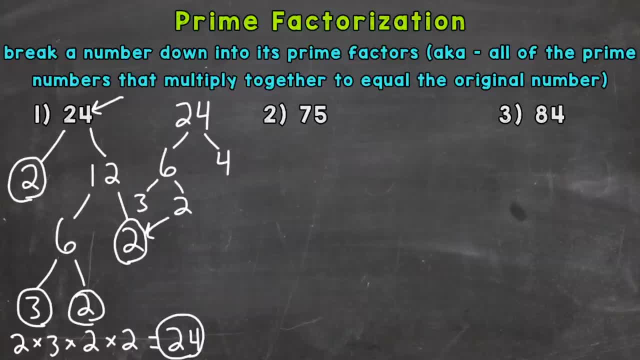 Well, 3 and 2 here for 6, factors of 6.. And then 4 would be 2 and 2.. So we get 3,, 2,, 2, and 2.. So the same exact answer, but a different path. 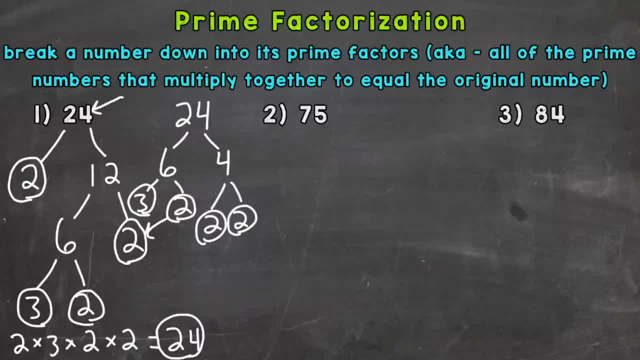 And in number 2, where we have 75. So we need to think of a couple of factors here to begin breaking this down to its prime factorization. Well, we know, 3 times 25 equals 75. So 3 and 25. 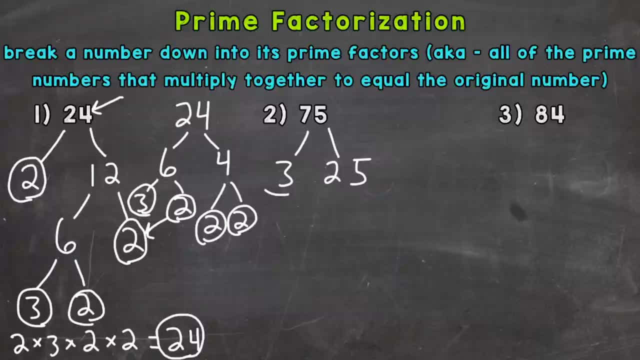 are factors. Now, 3 is a prime number, So the path ends there as far as that goes. But 25 is composite Factors of 25,, well, 5 and 5.. 5 is prime, So we are done: 3, 5, and 5.. So 3 times 5 times 5.. 3 times 5 is 15, times 5 is 75. 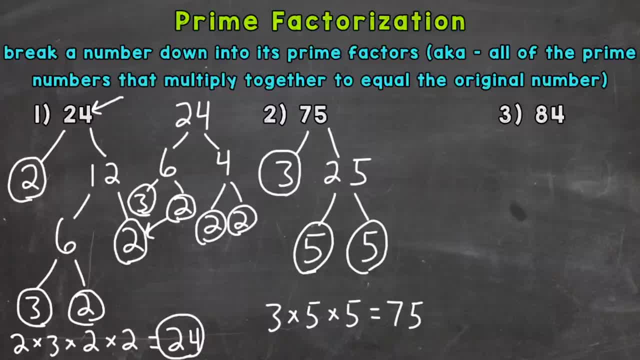 So we are correct as far as that prime factorization of 75.. Lastly, number 3, we have 84. So let's think of two factors here. Well, 84 is even, So we know 2 is a factor. 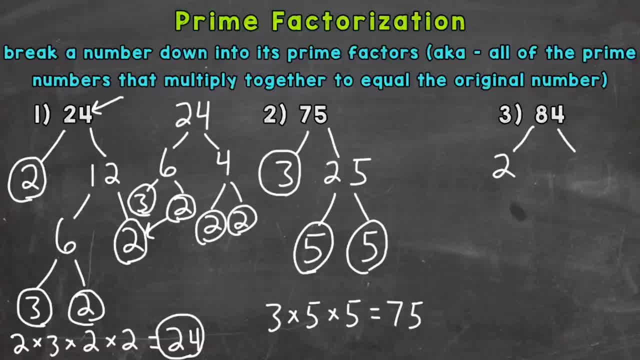 And it's going to be: 2 times 42 equals 84. So 2 and 42 are factors of 84.. 2 is prime. So we are done over there. We can circle it as we go, or at the end whatever works better for you, And then we 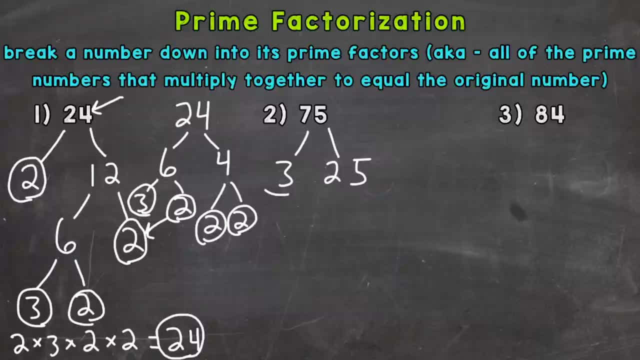 are factors. Now, 3 is a prime number, So the path ends there as far as that goes. But 25 is composite Factors of 25,, well, 5 and 5.. 5 is prime, So we are done: 3, 5, and 5.. So 3 times 5 times 5.. 3 times 5 is 15, times 5 is 75. 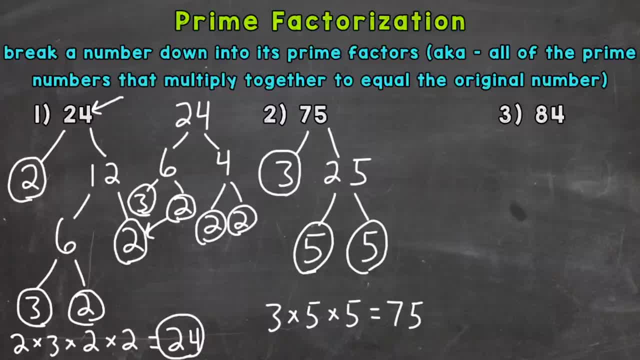 So we are correct as far as that prime factorization of 75.. Lastly, number 3, we have 84. So let's think of two factors here. Well, 84 is even, So we know 2 is a factor. 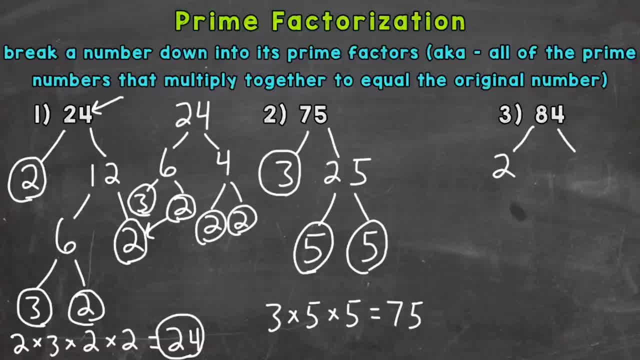 And it's going to be: 2 times 42 equals 84. So 2 and 42 are factors of 84.. 2 is prime. So we are done over there. We can circle it as we go, or at the end whatever works better for you, And then we 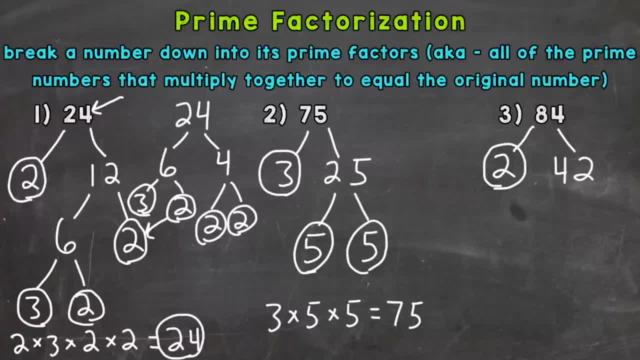 have 42. Well, 42 is composite. We know: 6 times 7 equals 42. So 6 and 7 are factors of 42.. 7 is prime, So we are done there, But 6 is composite, So we can continue on. We know 3 and 2. 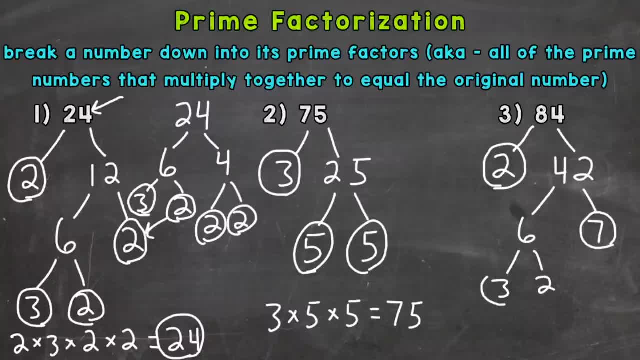 are factors of 6. And both of those are prime. So we have the prime factorization of 84. And let's double check. So we have 2 times 3 times 2 times 7.. Well, 2 times 3 is 6, times 2 is 12.. And 12 times 7. 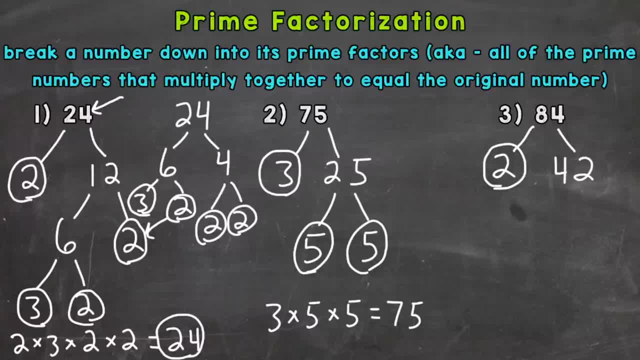 have 42. Well, 42 is composite. We know: 6 times 7 equals 42. So 6 and 7 are factors of 42.. 7 is prime, So we are done there, But 6 is composite, So we can continue on. We know 3 and 2. 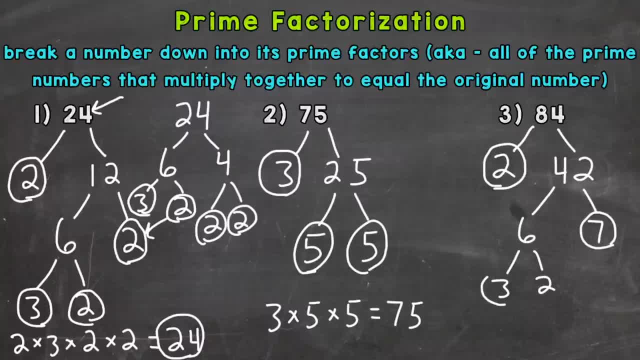 are factors of 6. And both of those are prime. So we have the prime factorization of 84. And let's double check. So we have 2 times 3 times 2 times 7.. Well, 2 times 3 is 6, times 2 is 12.. And 12 times 7. 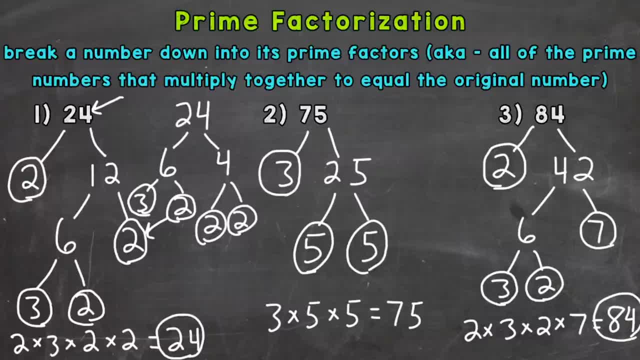 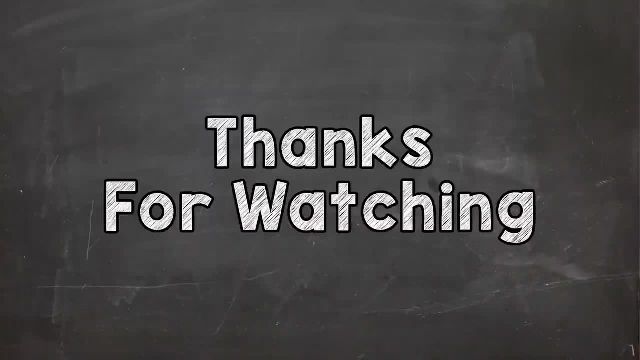 is 84.. So we have the correct prime factorization. So there you have it. There's how you find the prime factorization of a number. I hope that helped. Thanks so much for watching. Until next time, peace. 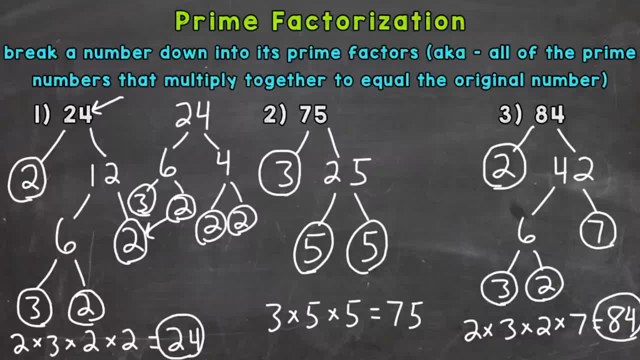 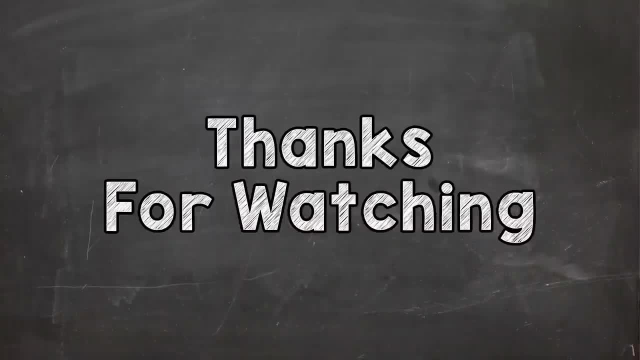 is 84.. So we have the correct prime factorization. So there you have it. There's how you find the prime factorization of a number. I hope that helped. Thanks so much for watching. Until next time, peace. 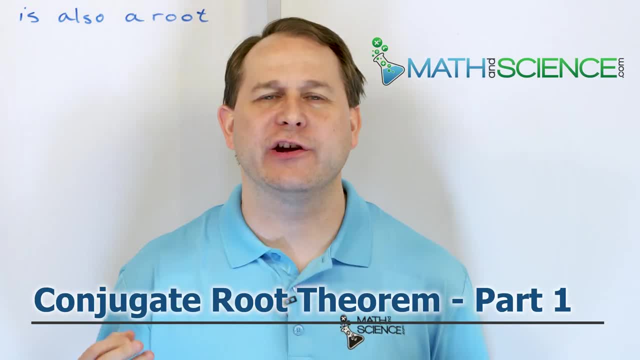 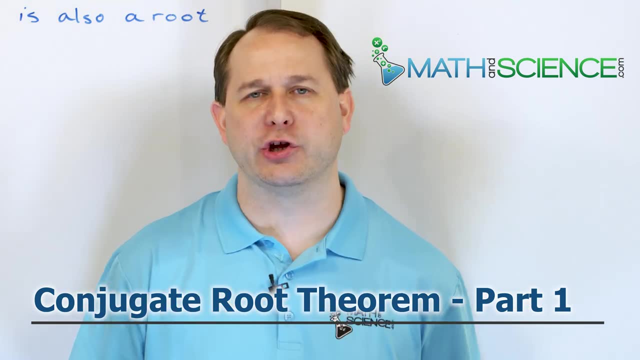 Hello, welcome back to Algebra. The title of this lesson is called the Conjugate Root Theorem. This is part one of two, So I said we're going to be covering some kind of random theorems that deal with polynomials. They're all really important. None of them are very hard to understand, but we 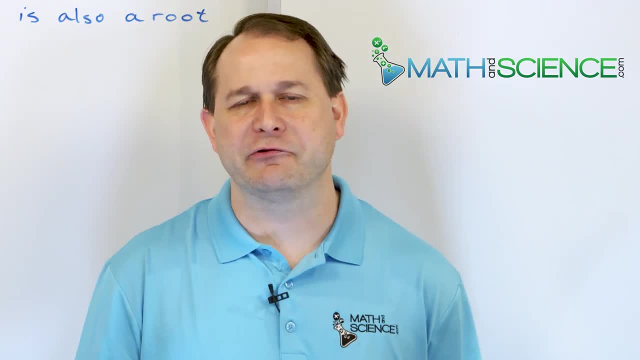 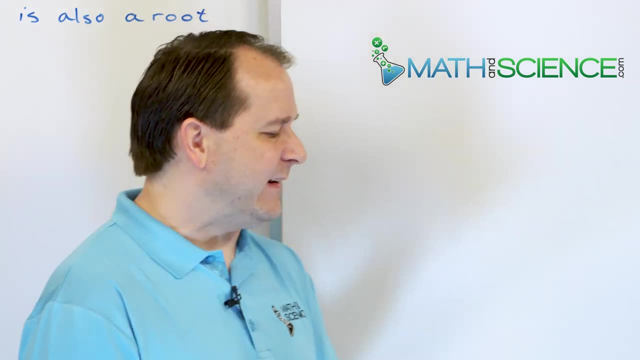 have to cover all of them. This one is called the Conjugate Root Theorem and actually you already know what it is, because I've told you through examples, but we haven't formalized it as a theorem. So here are the basic ideas. between these theorems- There's actually two theorems- 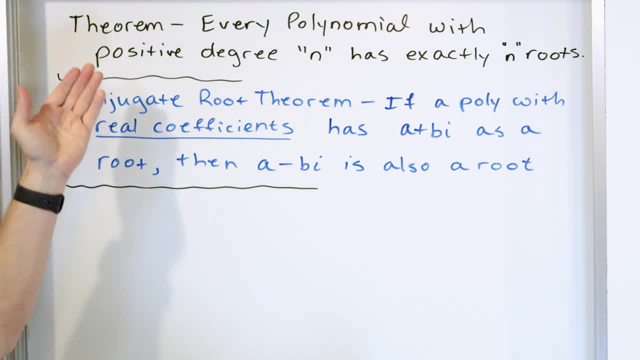 that we need to learn, both of which you already actually know. The first one is really an untitled theorem. It says that every polynomial with positive degree n has exactly n roots. So that's something that we've been telling you from the very beginning. That's just a theorem. 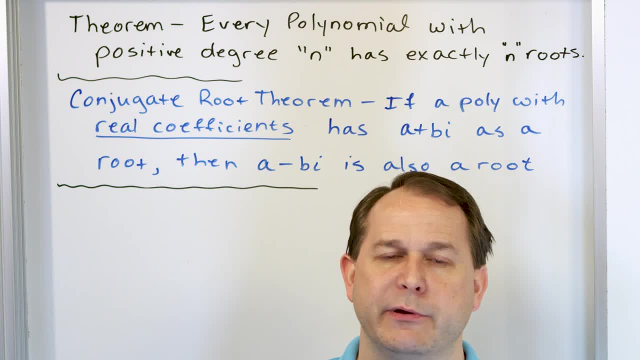 that's formalized, as it is true, for every polynomial has a positive degree. The degree of the polynomial tells us how many roots it has, and you already know this. Think of a line: mx plus b, So 3x plus 4, for instance. That's the equation of a line. What is the degree? 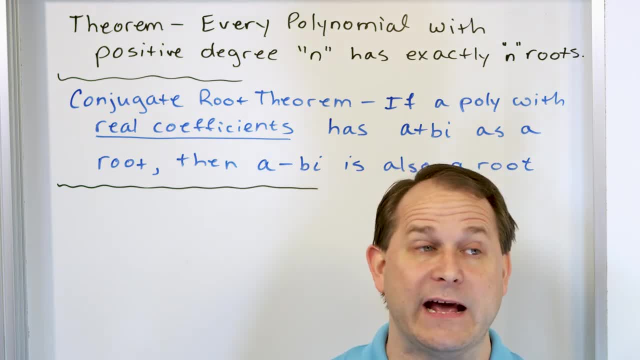 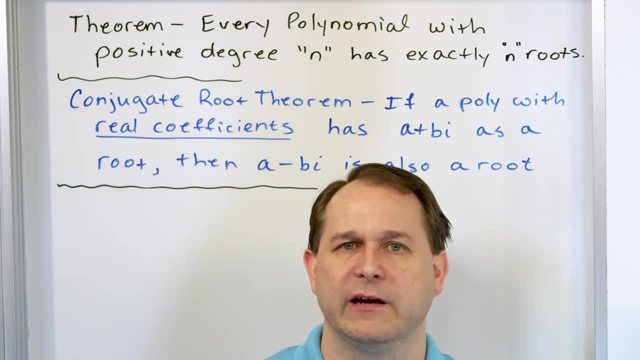 of that equation, The degree is 1 because that line has x to the first power, right? This thing tells you that every polynomial- and, yes, a line is a polynomial, it's just a degree of 1, has exactly n roots. So it tells us that a line has a degree 1.. It should only have one root. 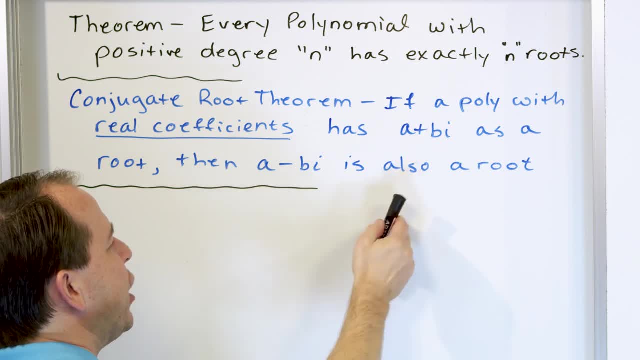 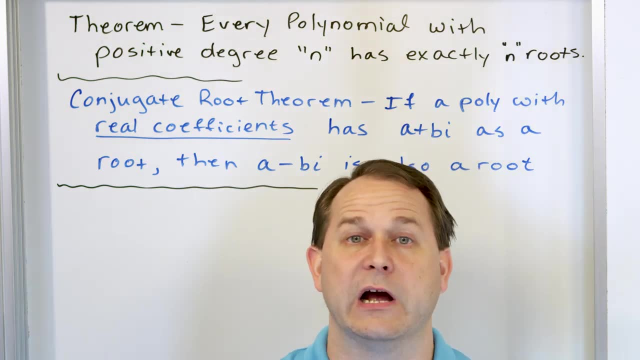 And if you think about it, if a line goes slanted like this, it can only cross the x-axis in one location. Of course there are special lines that are horizontal. They don't have any roots because they're special horizontal lines. But for every other line you have to have a degree of 1. So